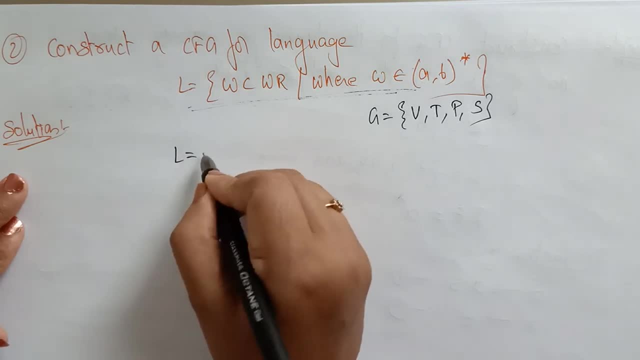 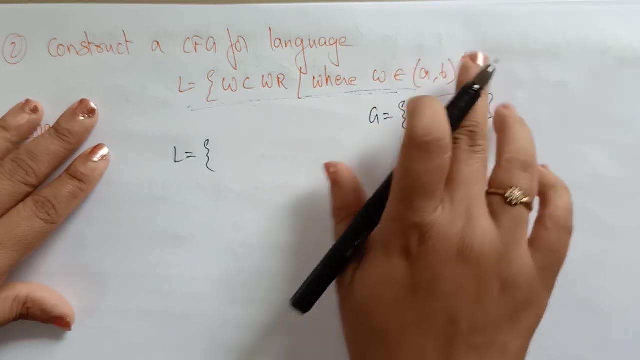 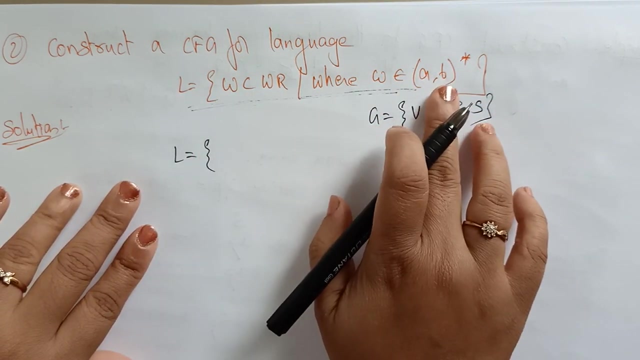 a given language, l. Okay, so this is the l, the language, This w. whatever the w that is there, that w is belongs to ab, ab multiples, ab star. they are given ab multiples. are there? Means w that is a string belongs to a, b, a, b, b and a, b, a, b, b, a, b a. So like that it's a multiple. 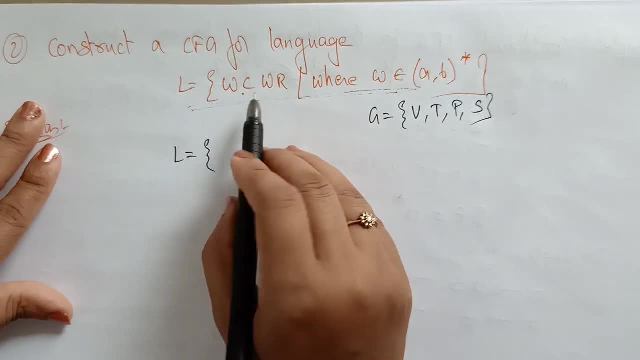 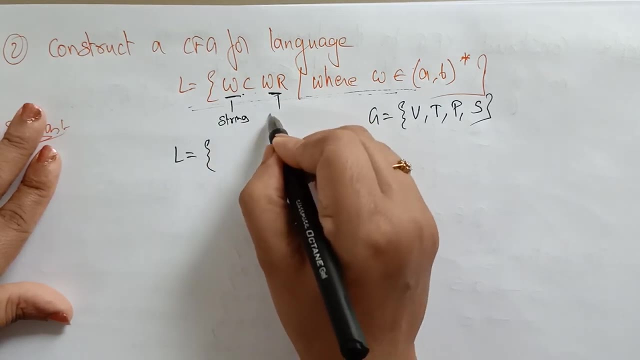 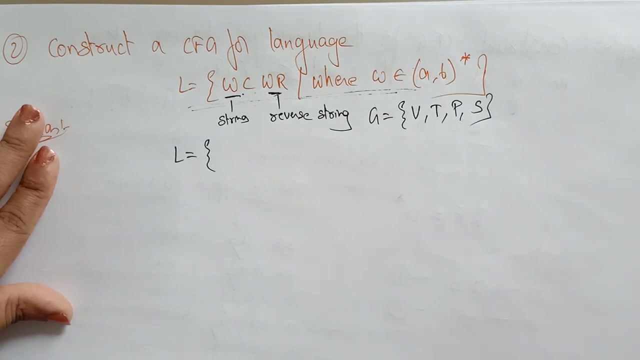 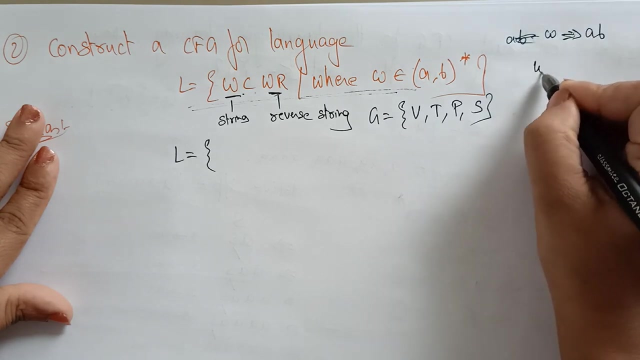 And c is the constant. Then what is this? w and wr? Okay, w is a string, wr is a reverse string. I already explained in the closure properties w reverse string can be represented as a wr. Suppose, if we get ab, w as ab, then wr is can be written as a ba. It's just reverse, Okay. 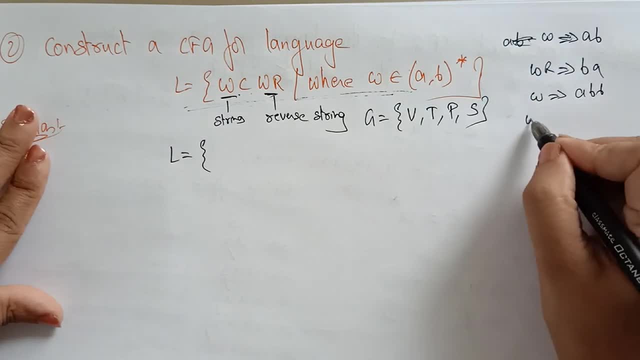 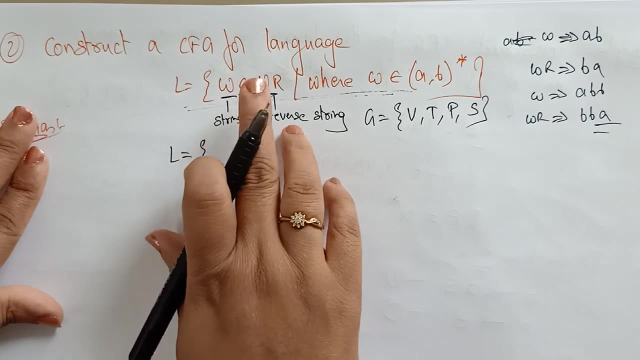 suppose if the w is a, b, then it can be written as a, b, a, It's just reverse. Okay, suppose if the w is a, b, b and the w are represented as b, ba, The reverse of the w. So here the string a, constant c. 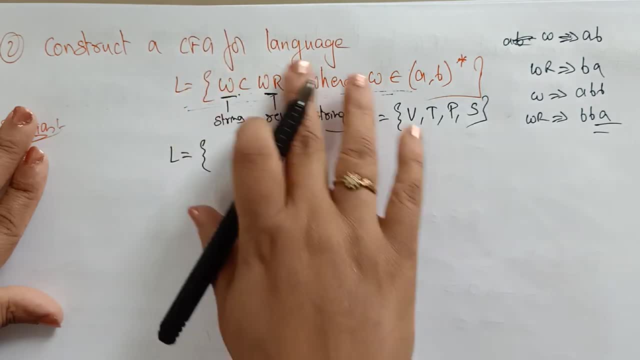 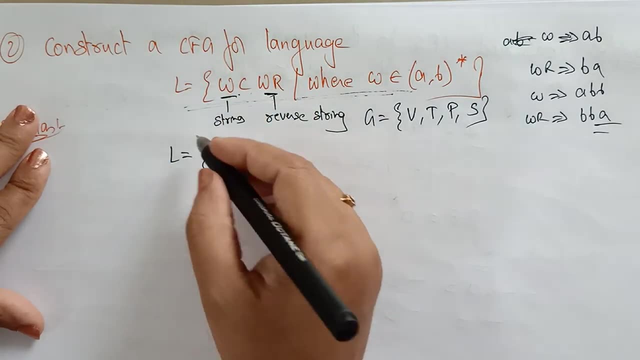 and the w are reverse string. The language is represented like this. So let me write the language strings that can be generated for the given language. Let me write the strings that you can generate for the given language. So in place of a, suppose I have written a, a Because 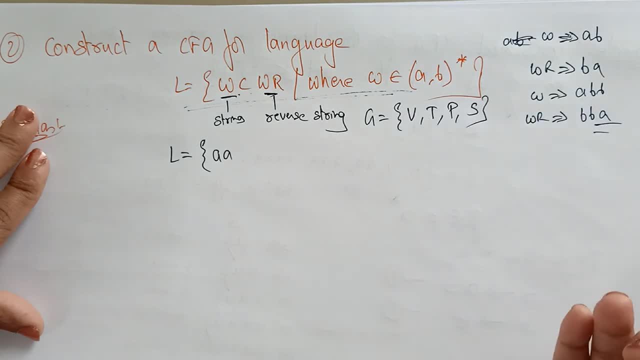 it is a, b is star, So I can write the string that can be generated for the given language. So in place of a, I can write any number of a's, including epsilon, So I can write any number of a's: a, a, c is. 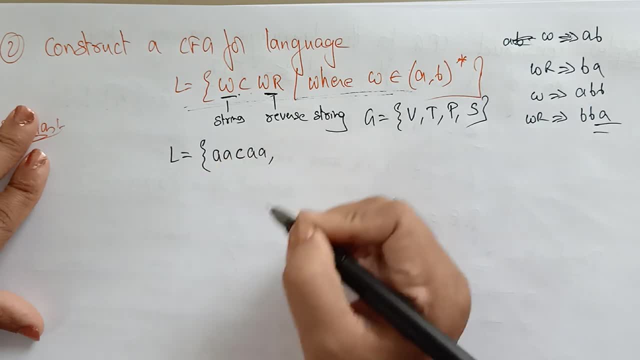 a constant and the reverse of a is simply a, a. And if I write b, a as a, b c is a constant. Reverse of b is b itself. Let me take a b This time, w I have taken as a, b c is the constant. What is the? 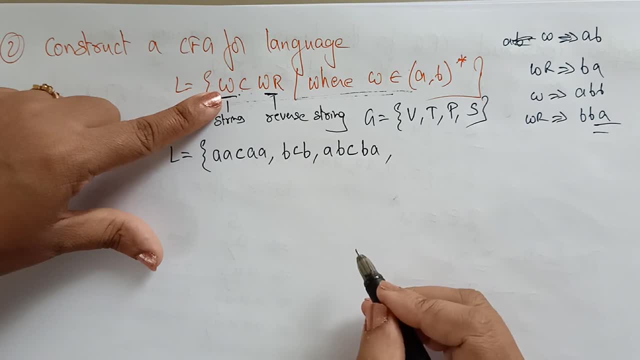 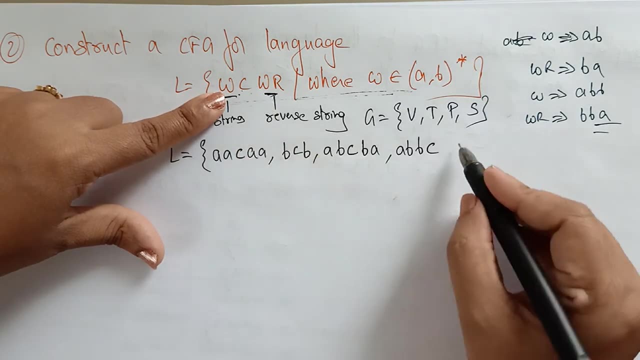 reverse of a, b, b, a. Okay, so suppose if I take a, b, I can write any number of a's including epsilon b, b, as w, c is. the constant Reverse of w is b, b, a. So in this way the strings can be generated. 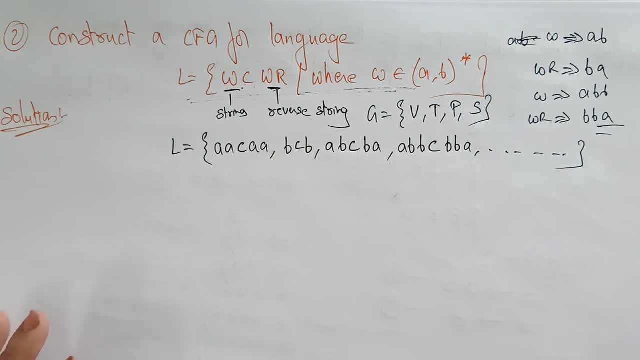 for the given language. Okay, the strings that can be generated for the given language. So now let me write the grammar, The production rule. I need to construct the context. free grammar. right, I have taken any of this input. These are the inputs. I have to take any one of the. 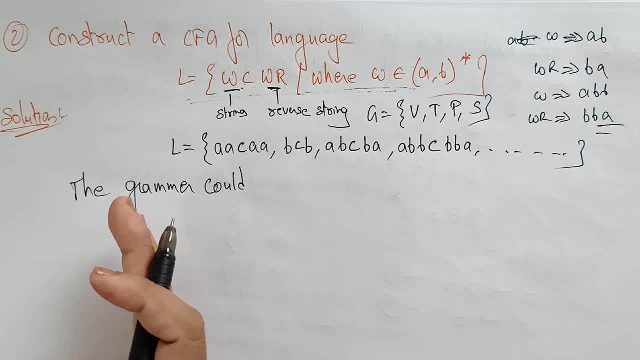 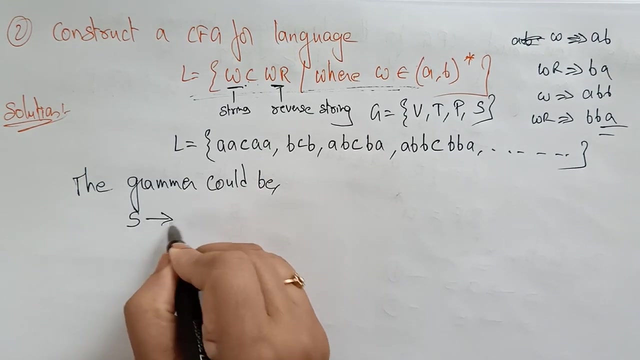 input and I have to derive this input by using the production rules. That is a context free grammar. Okay, by taking any one of the input. I need to derive that input. The grammar could be: what is the grammar? The grammar could be like: starts with the s symbol. 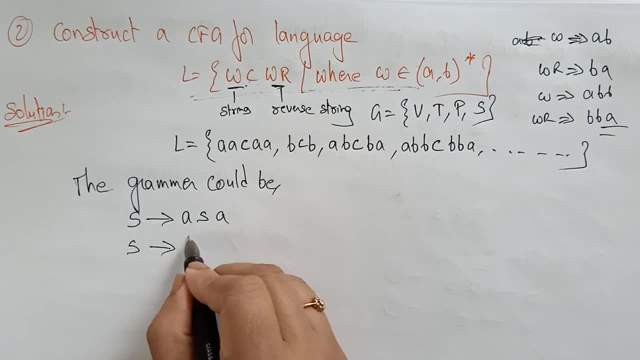 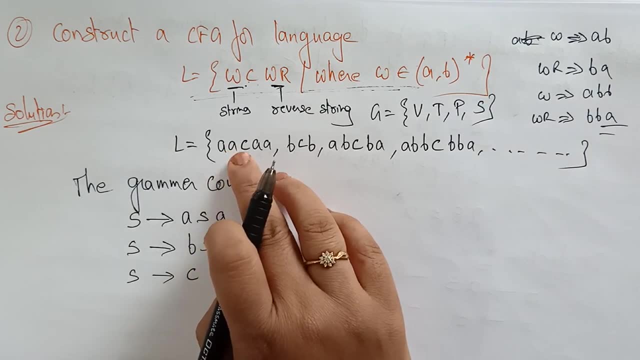 It can be a, s, a and s. it can be b, s, b and whatever the s that it should be the c constant, c, Okay. so starts with a, c, a. or it starts with b, c, a. Okay, here in the place of s, 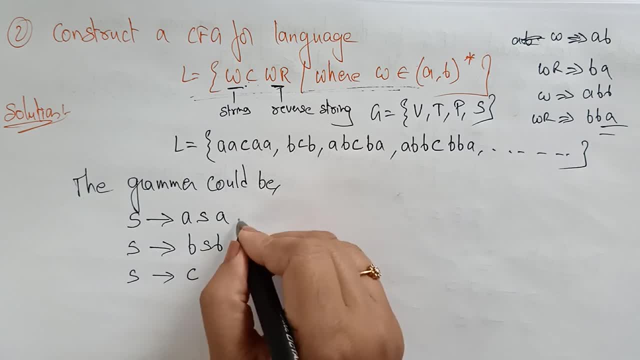 you can write a, b, c, a- Okay. so here in the place of s, you can write a, b, c, a. Okay, here in the place of s, you can replace with the c. So these are the production rules. We call it as a rule. 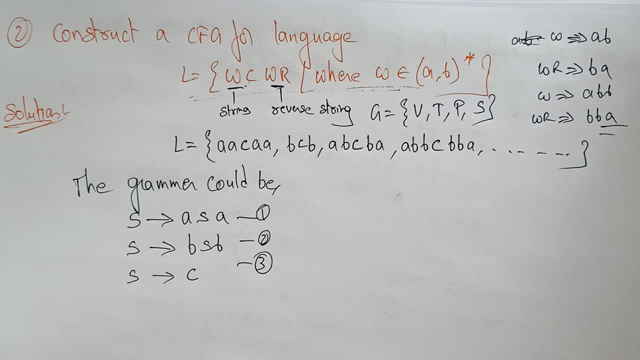 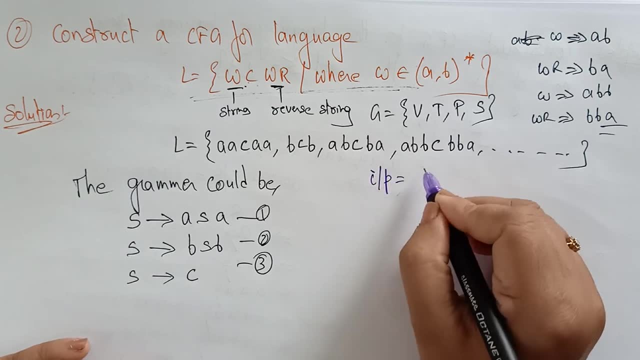 number one, two and the three. Now, okay, now, if you want to derive a string, let me take a string. That is the input. Let me take the string as a, b, b, c, b b a. I want to derive this string. 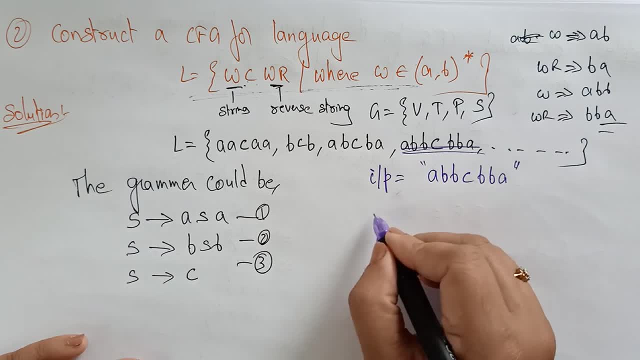 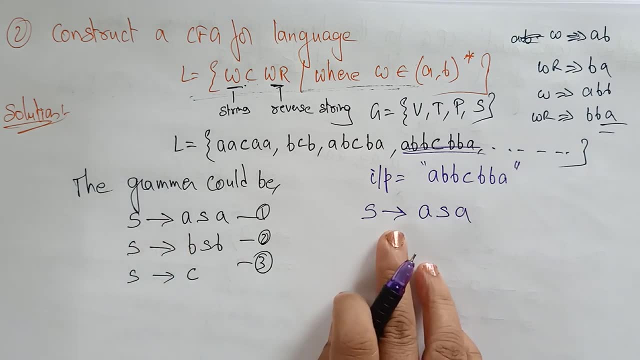 I want to derive. this input string Now starts with the start symbol. Okay, so start with the start symbol S determines a s a. Start with the start symbol s a s a. Okay, so now I am substituting in place of: 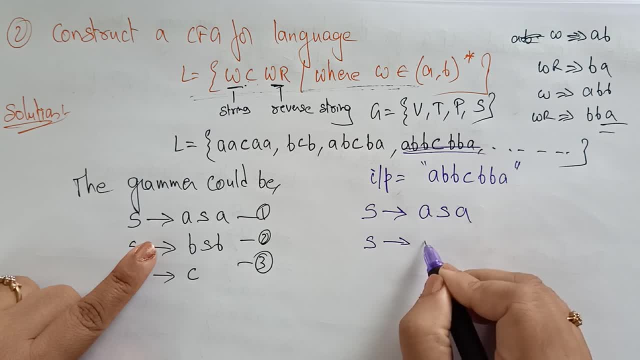 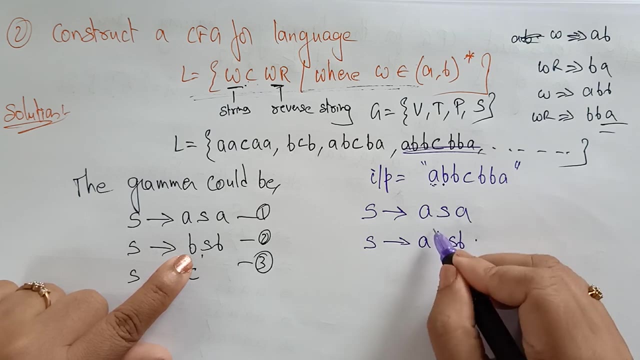 in place of s, I am writing next: what? what terminal you want? you want terminal b, So write the production. two. In place of s, I am writing b s b. and as it is a, So in place of a I have written b s b. So in place of a, I have written b s b. So in place of a, I have written: 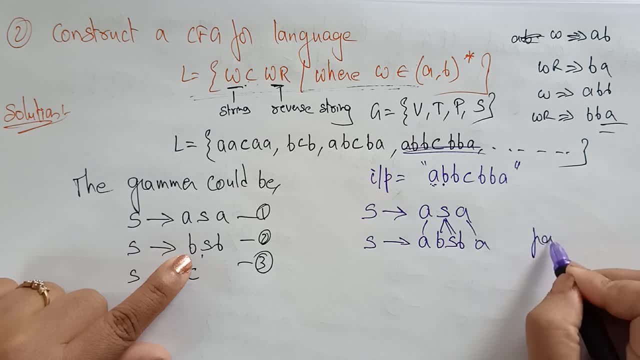 b, s, b. Okay, that is from rule two Now. so a, b is already a. terminals Now coming to the s. Okay, now I want the string. Next is also b, So next I want to. b means again, I have to replace.